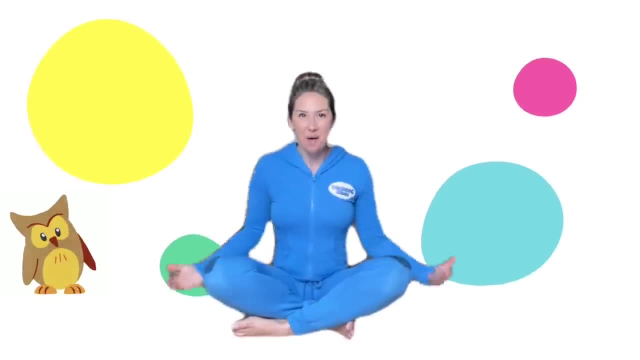 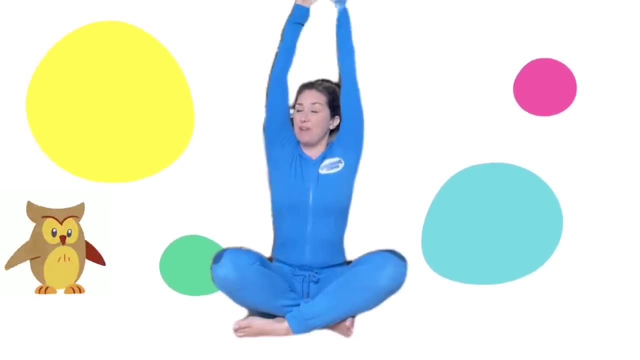 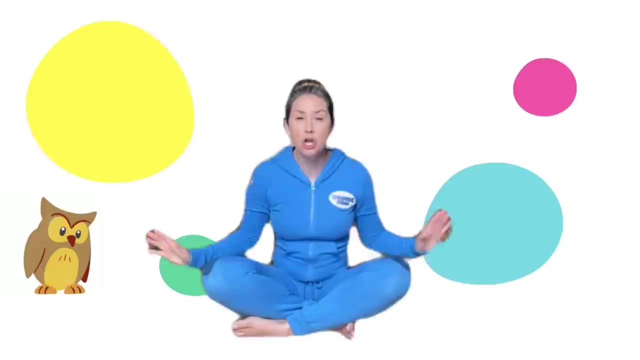 see us and say hello. it's an owl, Breathing in, lift and raise our wings to the sides and, breathing out, lower them back down and again breathing in, lift up, breathe out, lower down. She's found a hot air balloon in the forest and no one can. 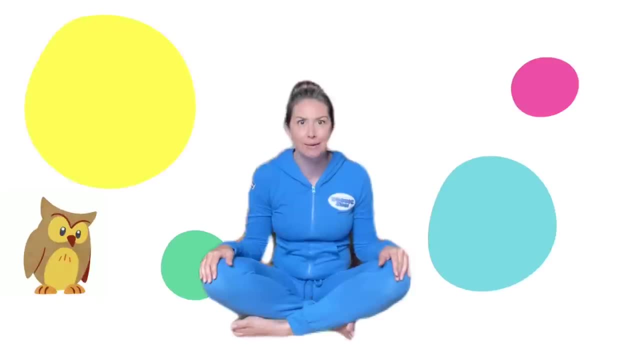 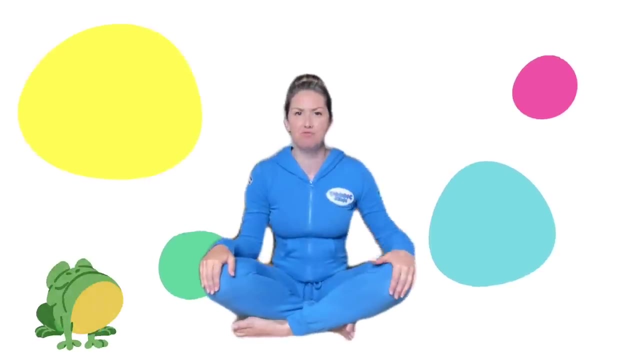 work out how to get it back up in the air again. Hmm, everyone comes to help and have a go. First the frog, who takes a big breath in, holds his breath, then does a big breath out and then holds his breath again. The frog likes the feeling of. 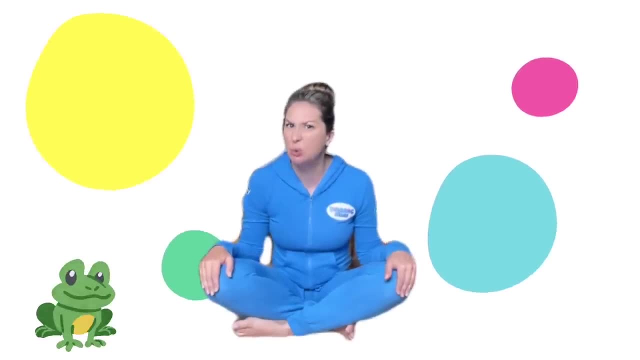 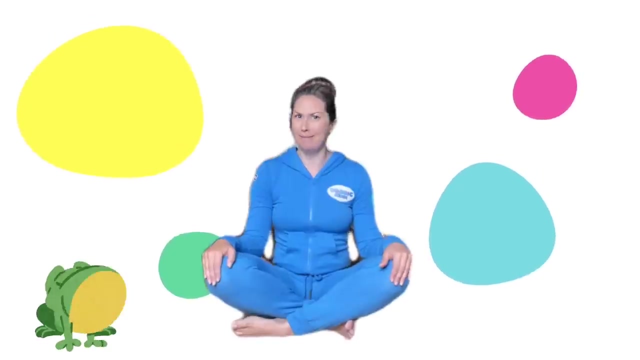 holding his breath and seems to like it. The frog seems to have forgotten about the balloon, so just does it all over again: A big breath in and hold it there, and a big breath out, and no breathing in for a few counts. That clearly isn't working to blow up the hot air balloon, but at least. 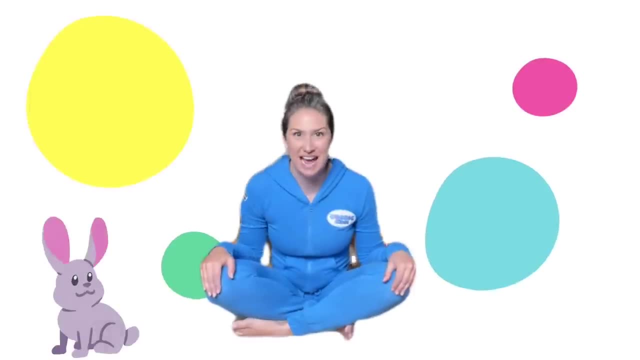 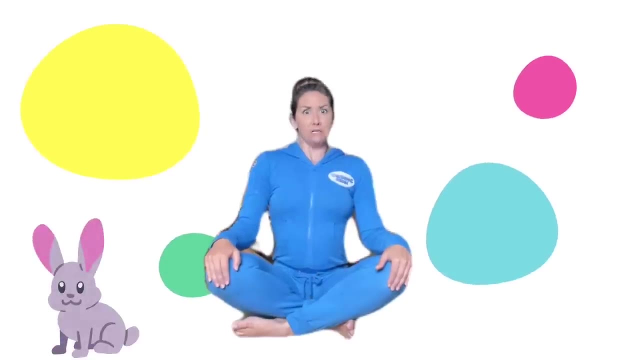 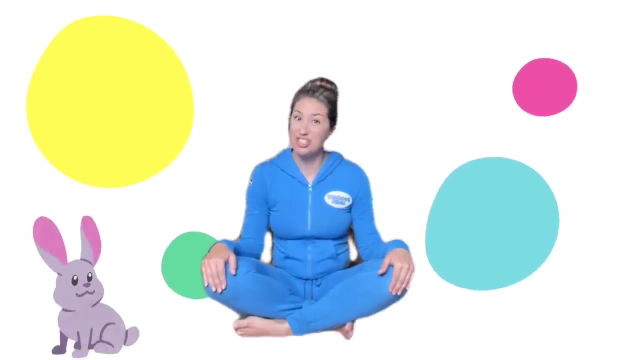 the frog enjoyed it. Next the bunny has a go, Doing a big breath in holding it, because the frog seemed to like that. Then an extra little bunny sniff to fill up to the top. She then lets her breath out through her mouth, which doesn't fill the balloon with much air. 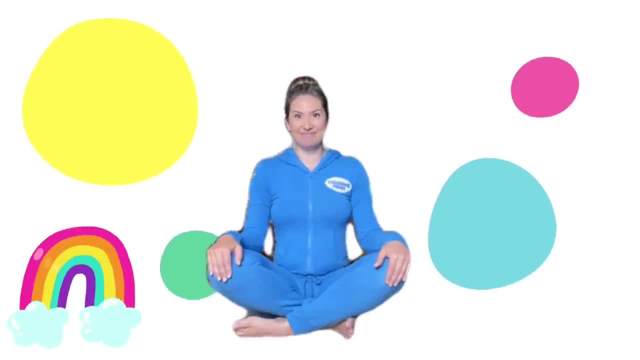 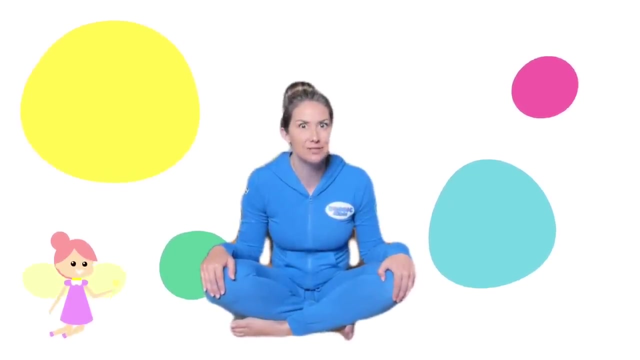 The rainbow tries next Copying the bunny, doing a big breath in A little extra sniff to add some more. Then, being a rather chilled out rainbow, just does a nice relaxed, long breath out. She takes a look, niet Still. 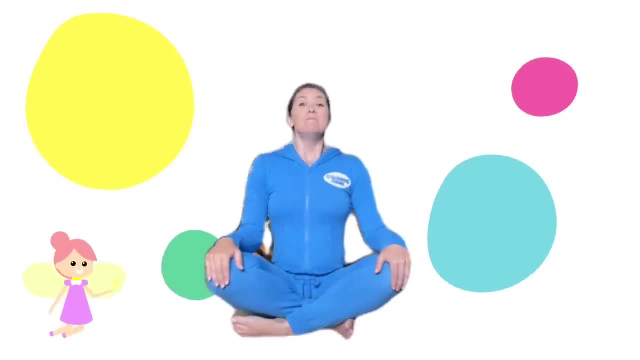 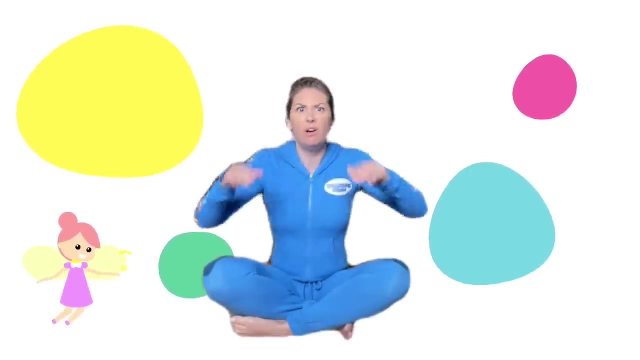 not making the balloon fill up…. Next to try is the fairy who thinks a special magic fairy dust wish could do the job, Taking a big breath in… a little bunny sniff for some extra Holding it… As we hold… out our hand with the magic fairy dust and now blow, But it doesn't do the job. 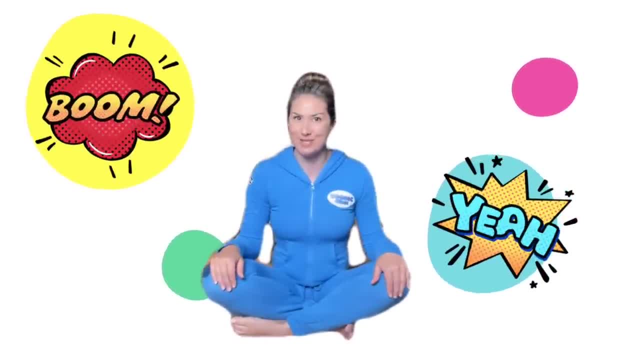 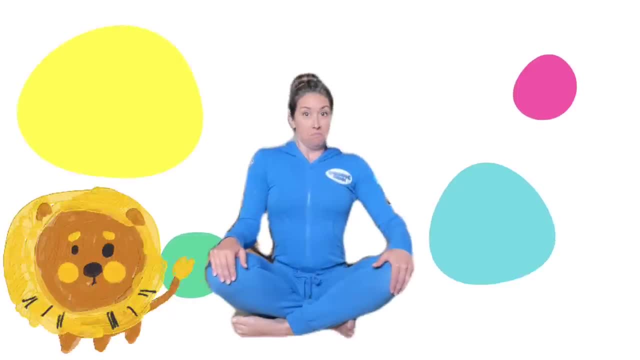 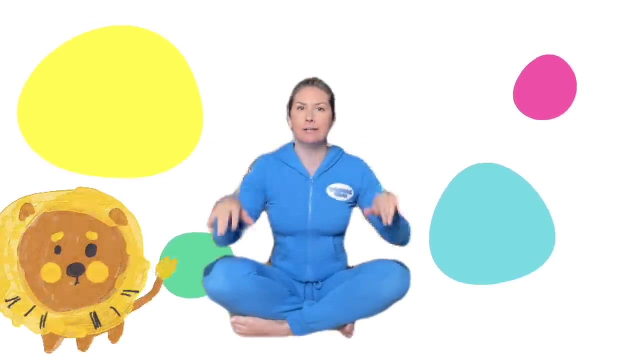 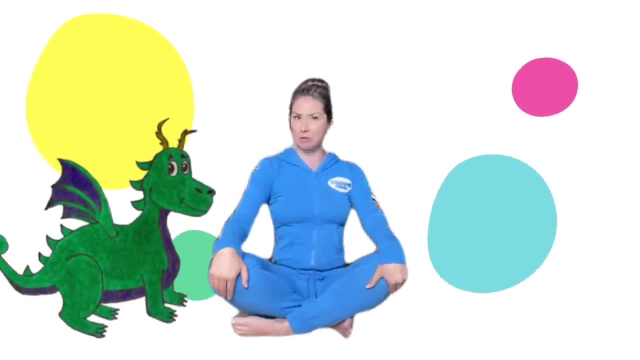 Next come the power puffers. First the lion breathing in, Sniff a little bit more, Hold, hold, hold, and then sticking out her tongue to do a huffy harry roar. Nope, that doesn't seem to work. Dragon has a go doing a big proud inhale. 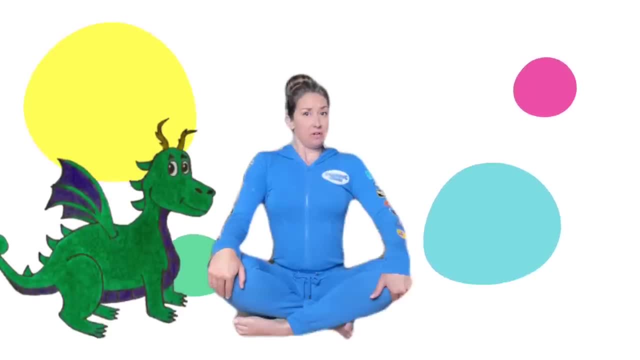 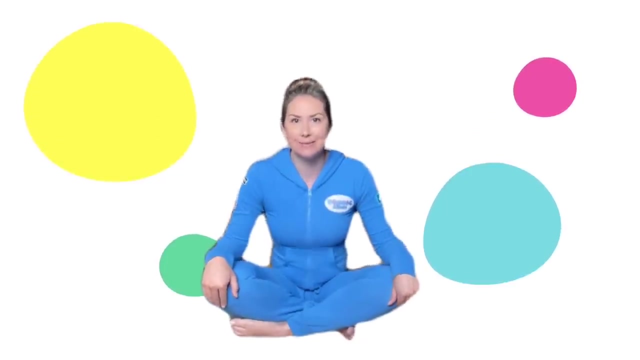 An extra sniff in to light the dragon fire and a big, fast puff which only seems to come out in smoke. None of them seem to be able to do it, or perhaps we can help To get ready. we take a moment to get our breath. 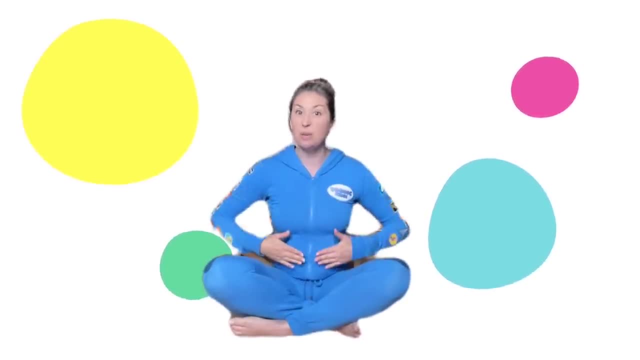 as deep and relaxed as it can be doing. our tummy breaths like the balloon is in there, right inside our tummy. Let's pop a hand on our tummies to help breathing in and out, and in and out and in. 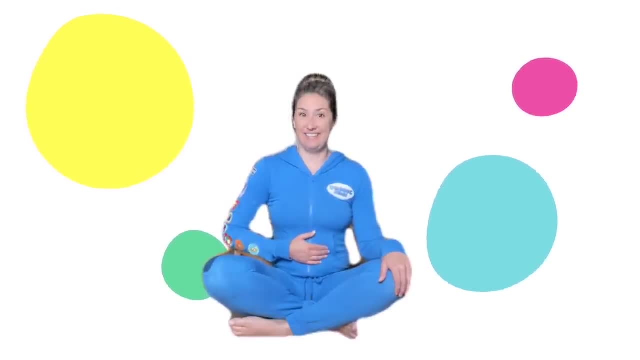 and out There. now our breathing engines are ready, Let's do our hot air balloon breath. It must be called that for a reason, right? We take a big breath in and that little extra bunny sniff for luck. Then we focus our breath, making an ooo shape with our lips. 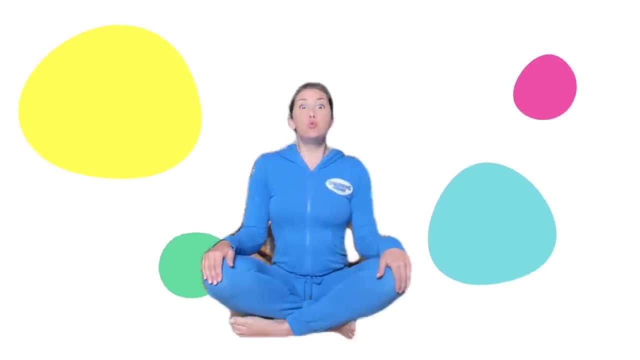 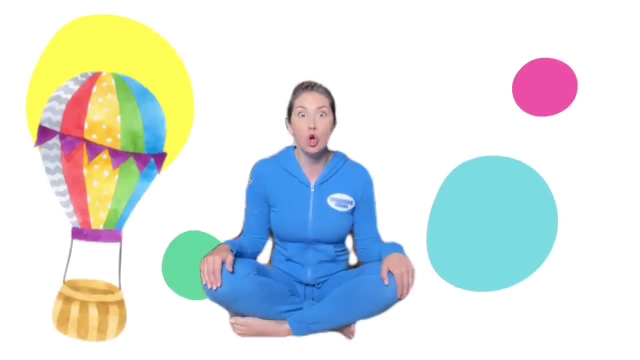 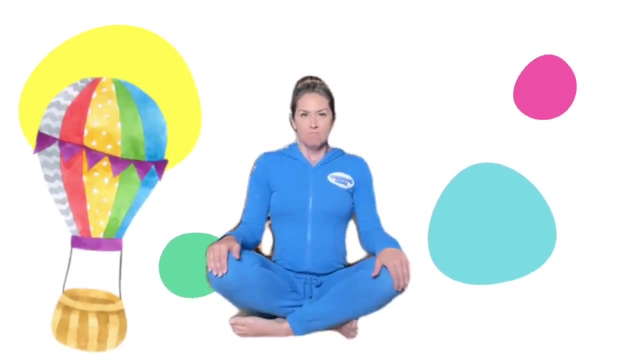 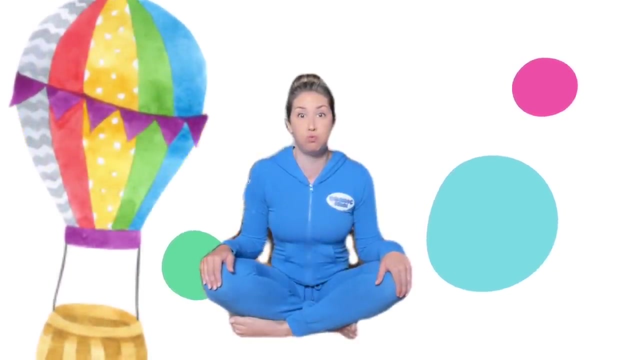 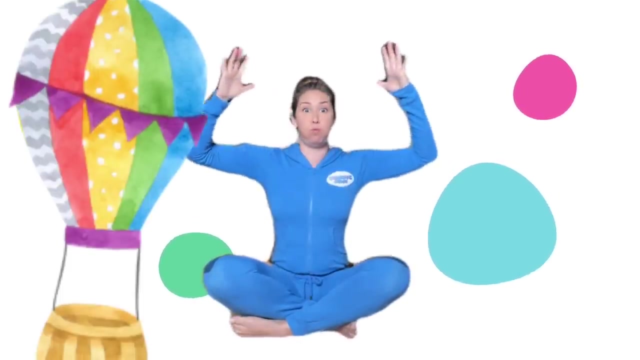 Here we go. Look as we blow, the balloon begins to fill up. Let's do some more. Breathe in big again and blow, And again in and blow. This time use your hand. It's getting bigger and bigger and bigger. One last one. 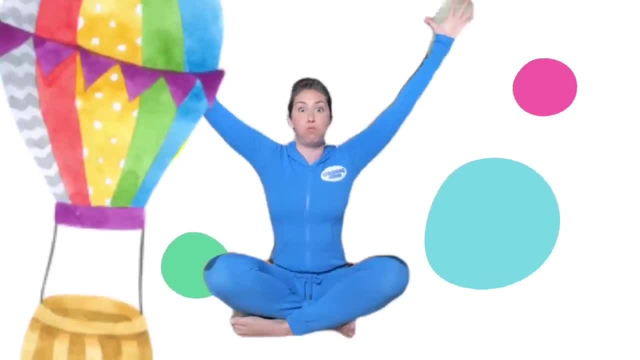 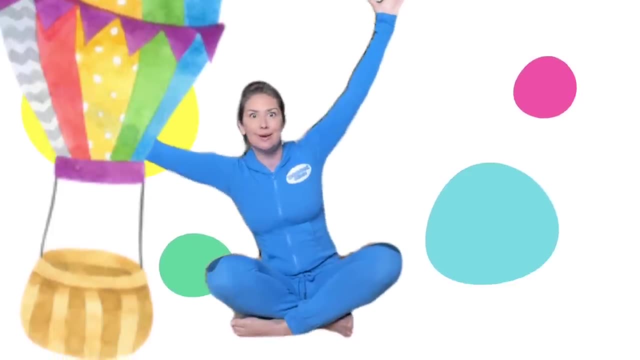 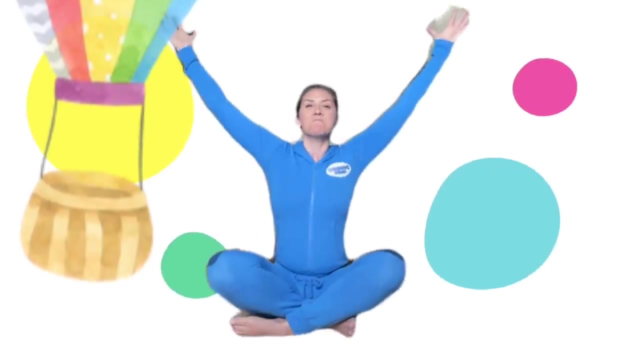 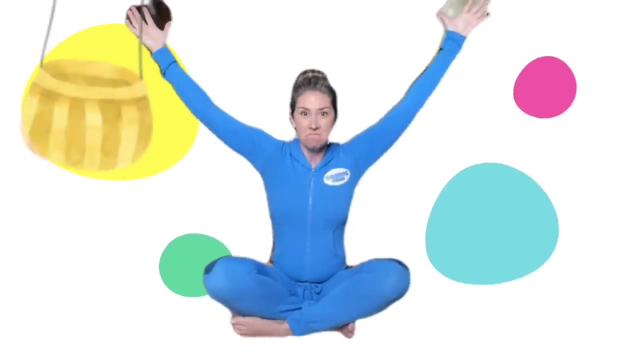 Breathe in and blow There. now it's as big as it can go and it's starting to float. Can we do another big breath to get it right up into the sky? Let's try Breathing in and blow, And in and blow. 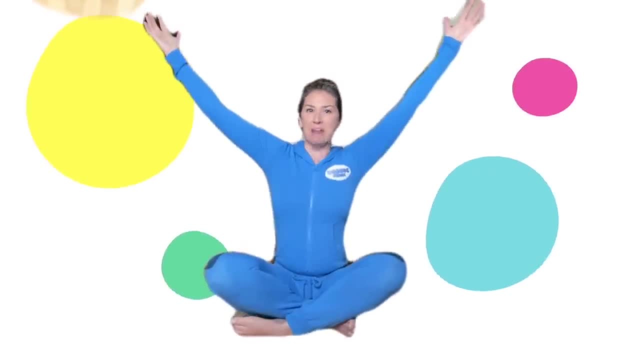 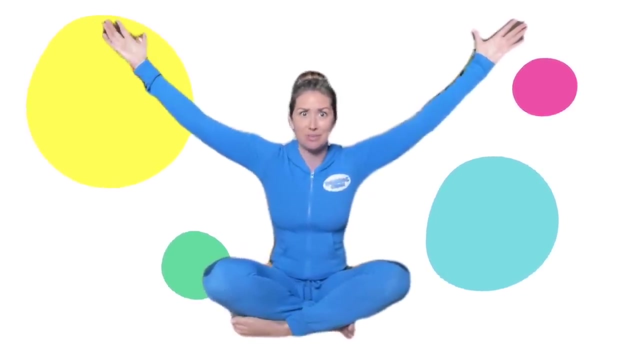 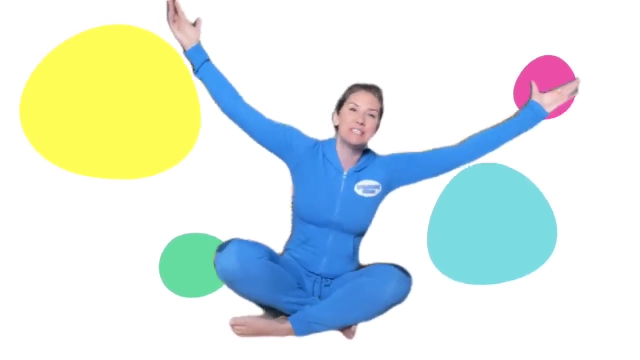 Oh, mind the trees. Breathe in and blow. Nearly there, Breathe in and blow. Wow, we did it. Quite a workout. We float up into the sky with the balloon rocking side to side, Feeling so peaceful and relaxed. 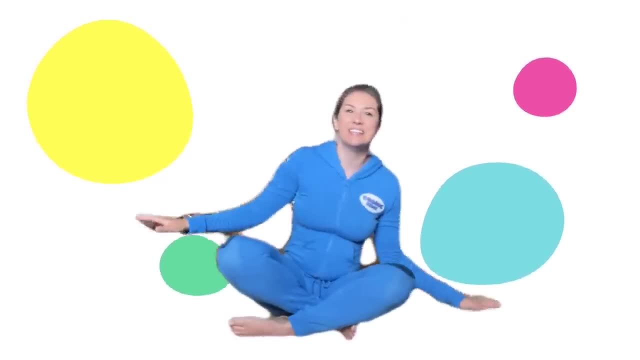 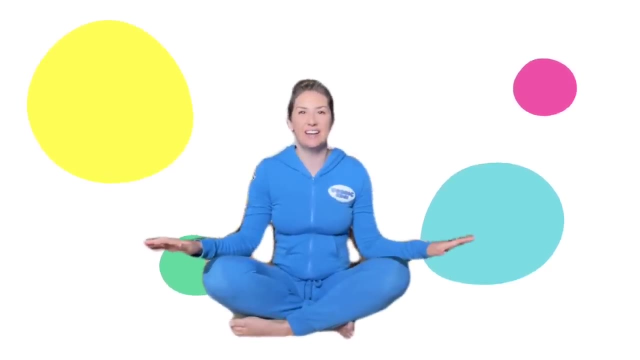 And we say our rhyme Tick tock like a clock until I found my centre. We found it And we sit in our centre spot here, Coming back to our tummy: breaths. Hold your hand on your tummy if it helps you, so you can feel it working. 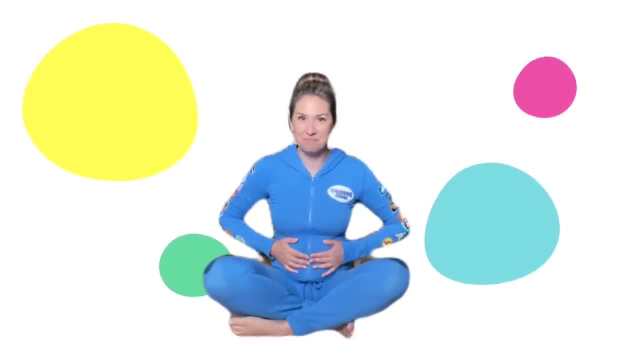 Quietly, Calming everything down, Filling it up, Emptying it out, Filling up and empty out, Feeling lovely and calm and relaxed. Well done you. Thanks for joining me on the breathing adventure. We really made a difference with our breathing. 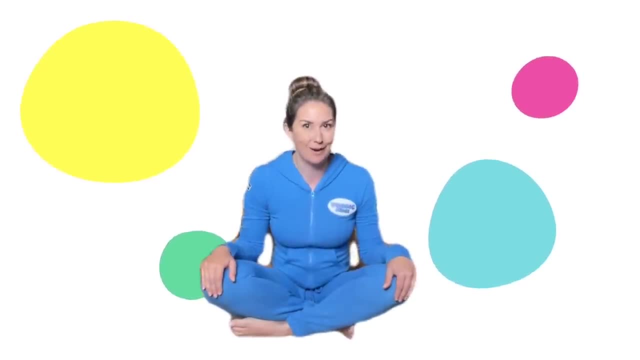 power today, And if you feel a little bit tired after that, then that's okay. Breathing with purpose and power like this takes strength and energy, But in doing so you give yourself more strength and energy by practicing. I'll see you again soon for more moving mindfulness and 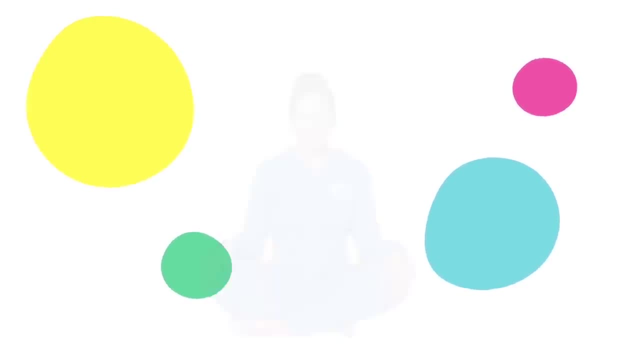 breathing. Thank you for watching. 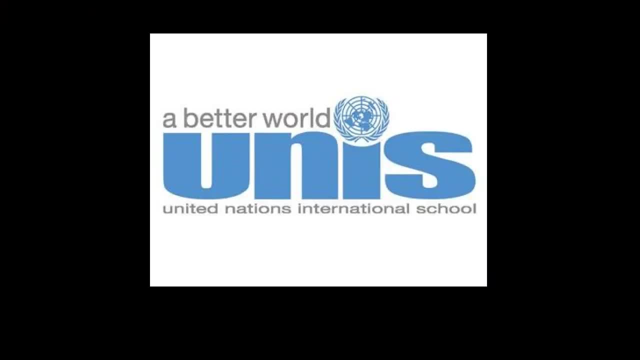 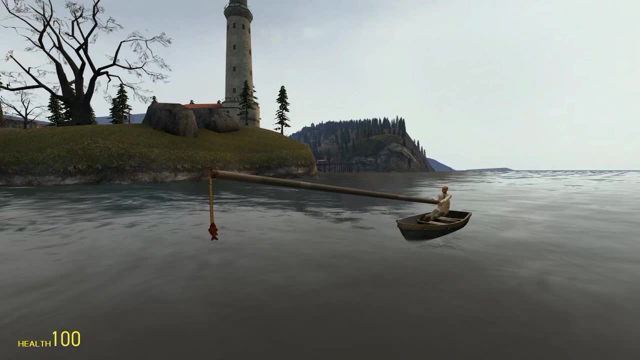 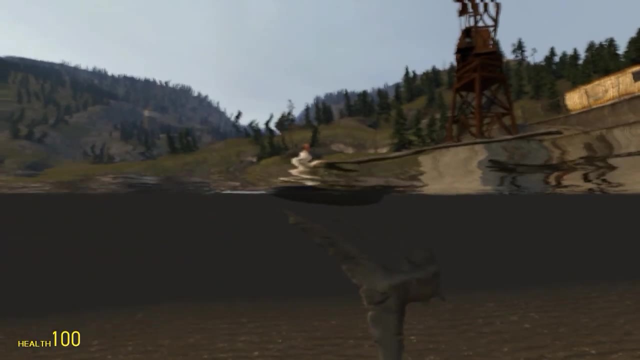 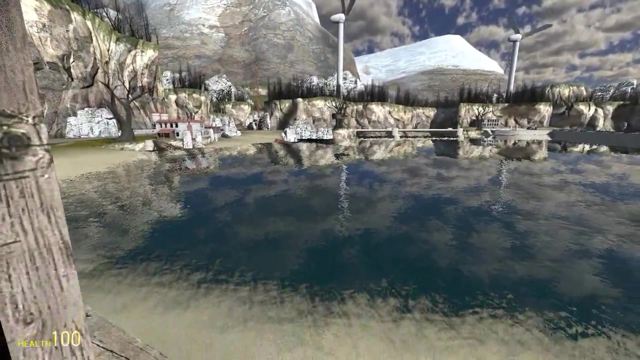 Ah, Dr Atkinson, having a nice day fishing Now. most aquatic life requires oxygen to be dissolved in the water in order for it to survive, But there are some situations where that oxygen level can be depleted. What a beautiful outlook. So raw sewage when it. goes into water will become oxidized, and thus removing oxygen from the water itself. Nitrate fertilizers will also encourage the growth of algae, which will reduce oxygen levels, as will phosphates that are used in many detergents for cleaning clothes- Algae. 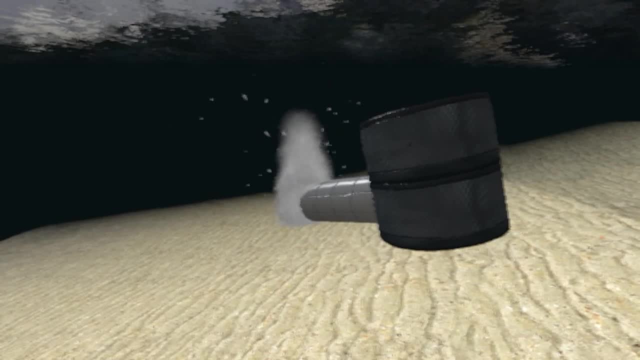 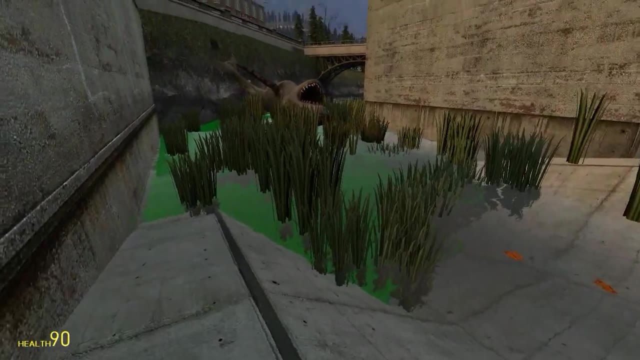 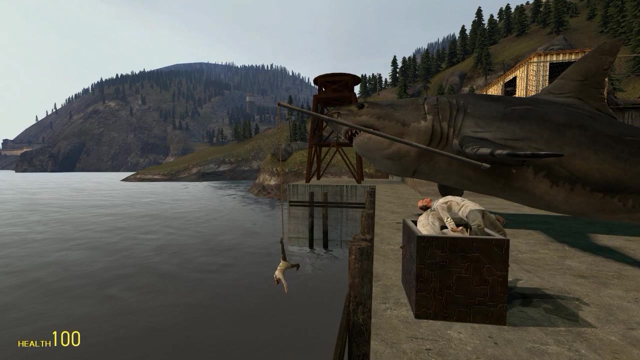 and other organisms will digest the phosphates, use up the oxygen, die and deplete oxygen levels even further, thus killing fish, who will suffocate as the algae will increase, die and sink and use up more oxygen as they decay. Well, that's unexpected. 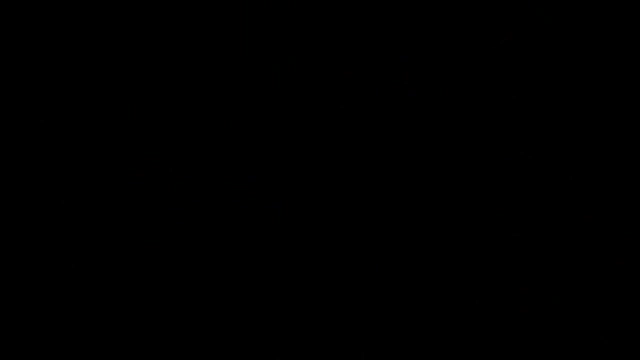 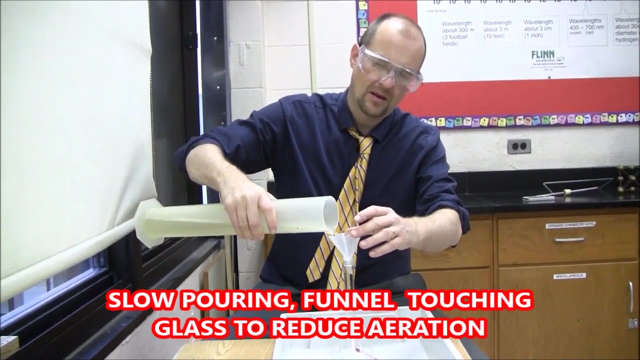 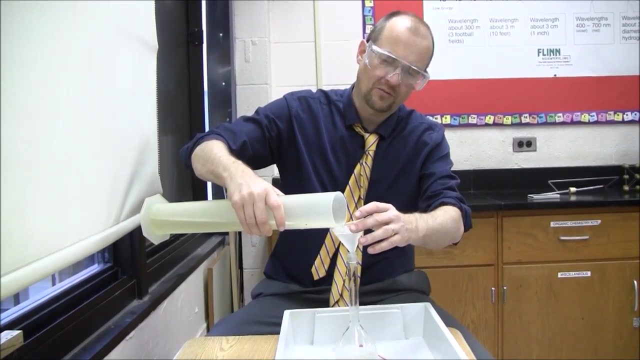 This is water from the East River of New York, So I'm going to put it into this container. Now you need to have a known volume of water. Now. this is a 250-millilitre volumetric flask, but I'm actually going to fill it up completely. It's going to be somewhere between 90 and. 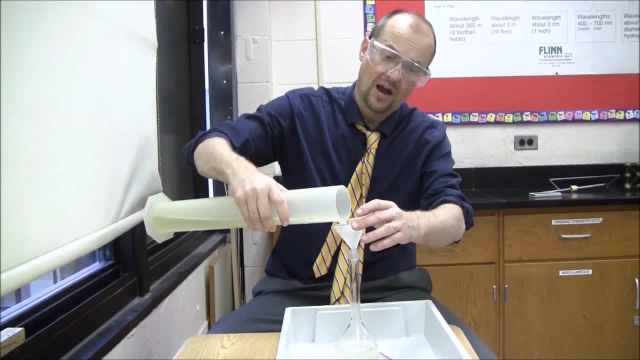 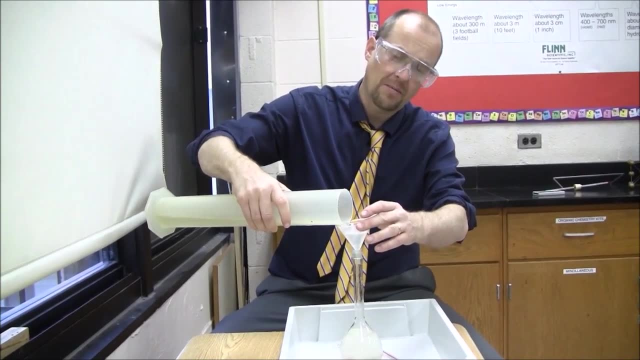 200 liters. completely it's going to be slightly more than 250, and I'm going to have to work that out later. I don't want to leave any air in the flask because of course then I'll be measuring the oxygen from the air and the water. I just want to measure it from the water.